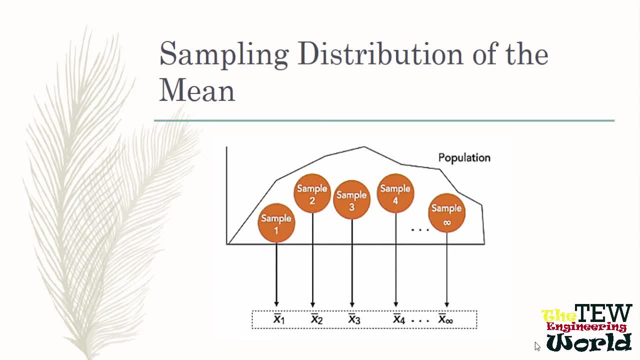 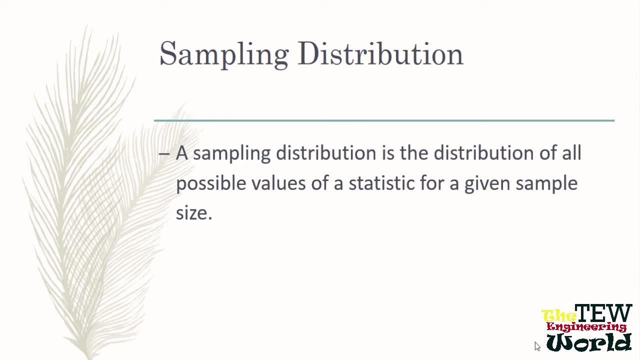 That set of means is the sampling distribution of the mean. So a sampling distribution is the distribution of all possible values of a statistic for a given sample size. The standard deviation of a sampling distribution is called the standard error, And this is a very important and useful definition in statistics. It is a term we encounter in many 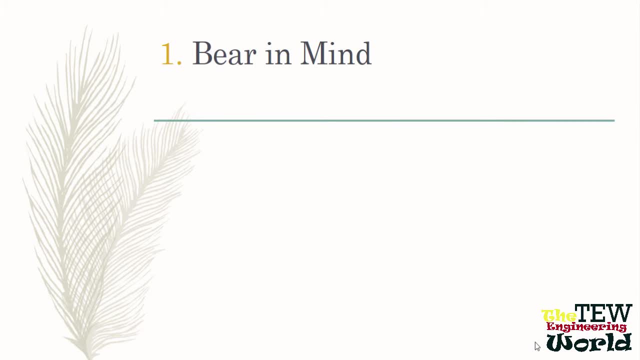 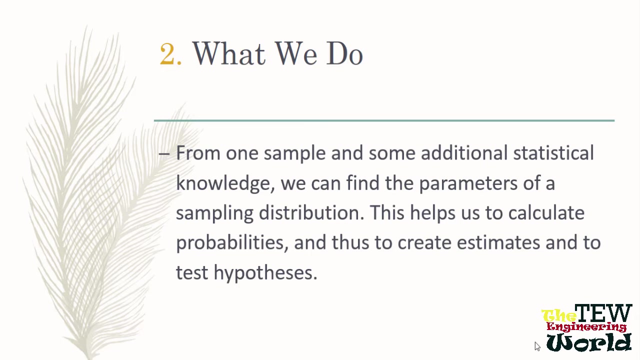 contexts. Bear in mind that when we do a study, we never actually create a sampling distribution. That would take an infinite amount of effort. Here is what we do: From one sample and some additional statistical knowledge, we can find the parameters of a sampling distribution. What does this enable us to do? 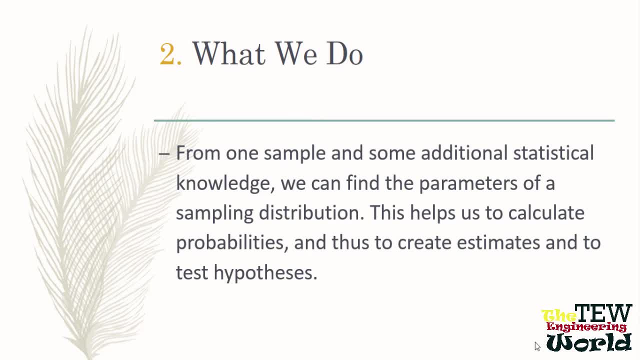 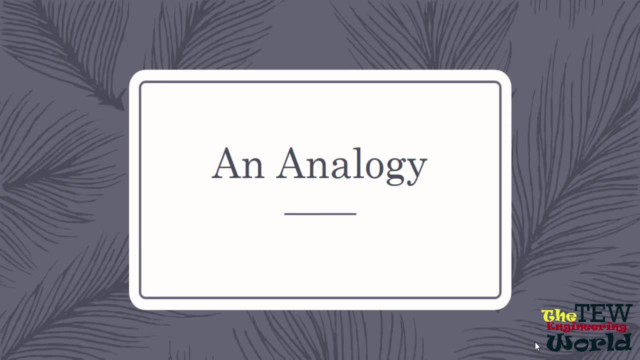 This enables us to calculate probabilities and thus to create estimates of parameters and to test hypotheses. Here is an analogy: It is something like a paleontologist working with a small fossil and recreating an entire dinosaur. In practice, step one is to calculate a statistic from 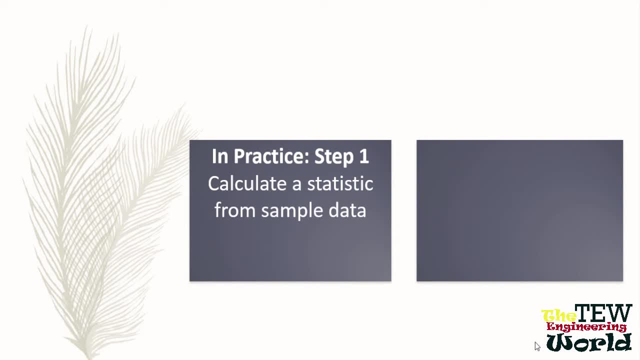 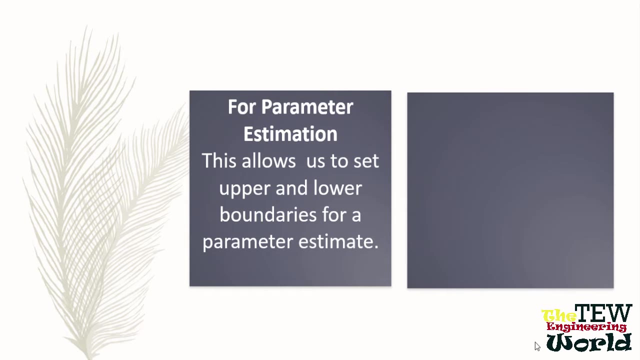 some sample data, And step two is to calculate a statistic from some sample data, And step two is to compare the statistic to the sampling distribution of the statistic for estimating parameters. What this enables us to do is set upper and lower boundaries for a parameter estimate. 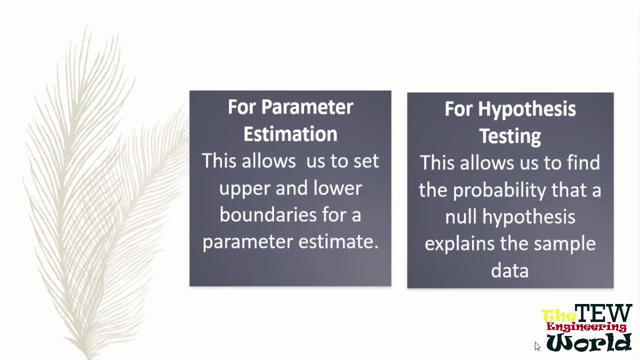 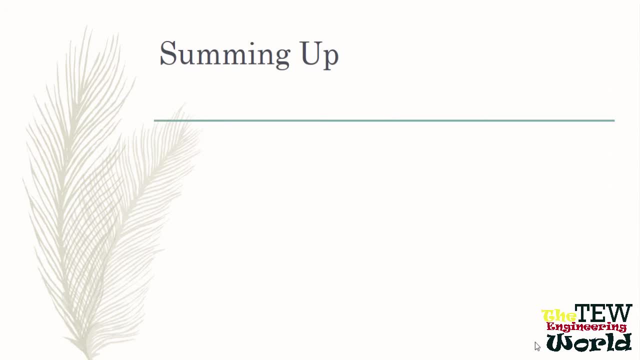 For testing hypotheses. this enables us to find the probability that a null hypothesis explains the sample data. In summation, a sampling distribution is the distribution of all possible values of a statistic for a given sample size. When we do a study, we don't create a sampling distribution. Instead, we use sample data. 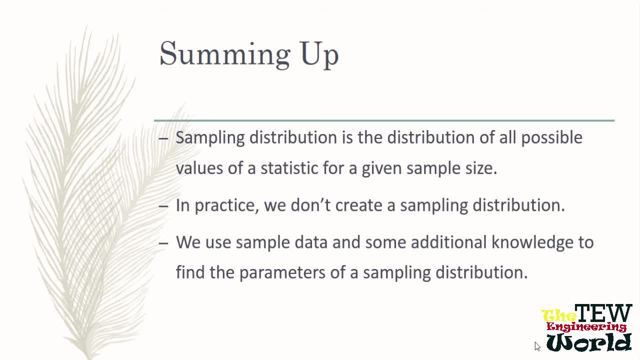 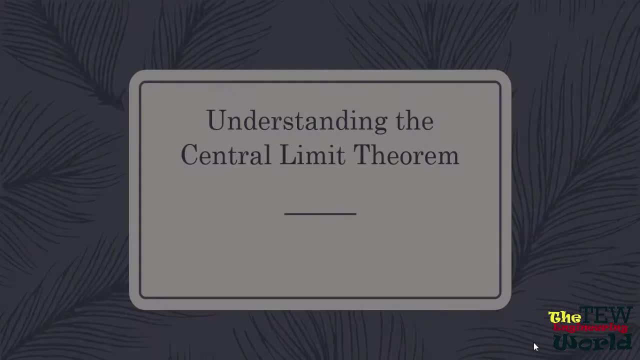 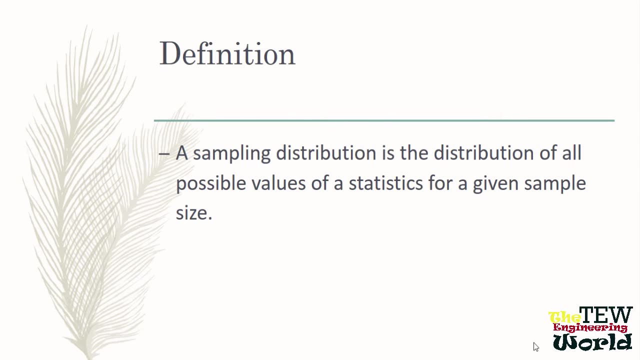 and some additional knowledge to find the parameters of a sampling distribution. Sampling distributions enable us to estimate parameters and to test hypotheses. Now we will learn about a very important statistical concept, the central limit theorem. We will start with this definition: A sampling distribution is the distribution of all possible values. 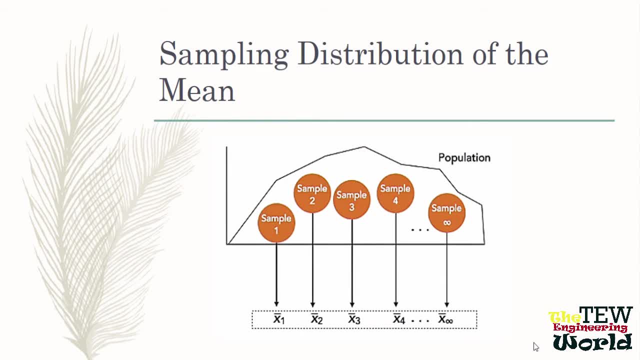 of a statistic for a given sample size. Here is a picture that shows what I am talking about: A huge number of samples coming out of a population. Imagine that each one has the same number of people and we measure each person on some attribute. We calculate a mean. 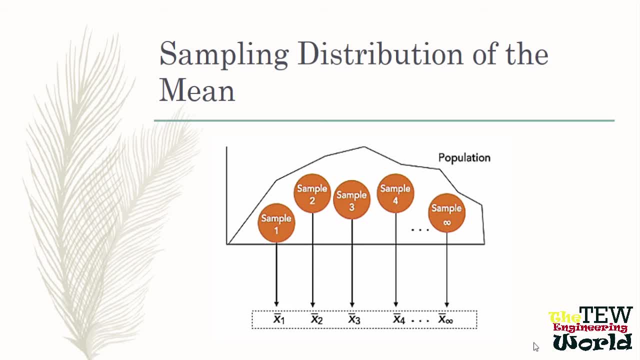 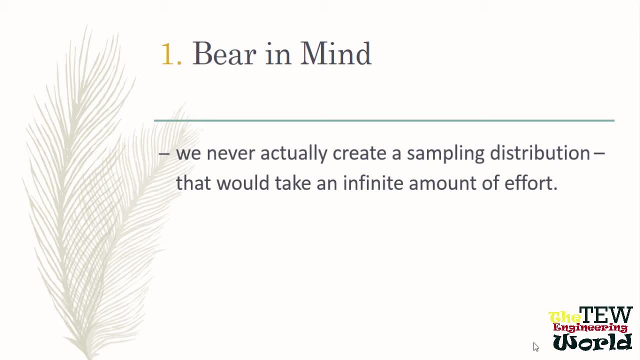 for each sample. That set of means is the sampling distribution of the mean. Now bear in mind that when we are doing a study, we never estimate the number of people. We never actually create a sampling distribution. that would take an infinite amount of effort. 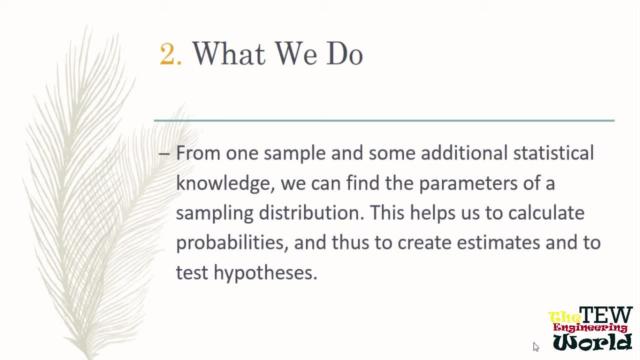 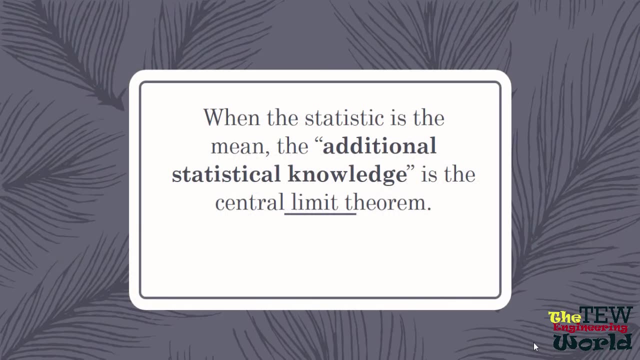 Here is what we do: From one sample and some additional statistical knowledge, we can find the parameters of a sampling distribution. What does this enable us to do? It enables us to calculate probabilities and thus to estimate parameters and test hypotheses. When the statistic is the mean, the additional statistical knowledge is the central limit. 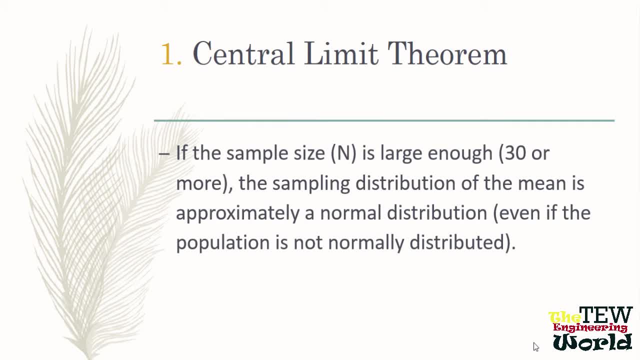 theorem, And here is the central limit theorem. If sample size n is large enough- 30 or more- the sampling distribution of the mean is approximately a normal distribution, And this is important even if the population is not normally distributed. The sampling distributions mean, mu, sub, x, bar. 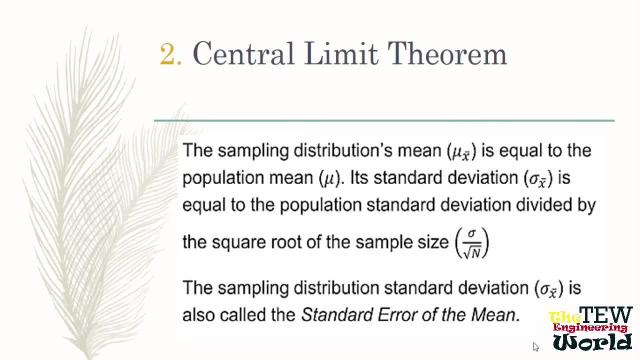 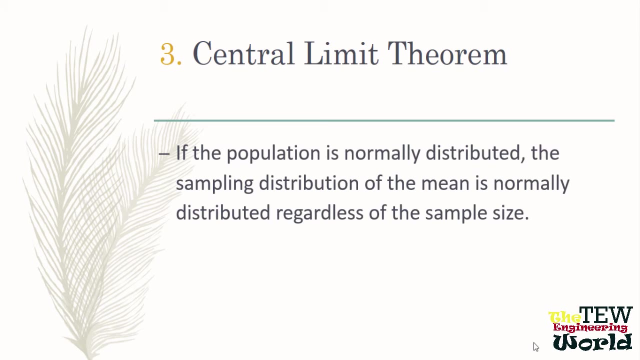 is equal to the population mean mu. Its standard deviation sigma sub x bar is equal to the population standard deviation divided by the square root of the sample size. The sampling distribution standard deviation sigma x bar is also called the standard error of the mean. If the population is normally distributed, the sampling distribution of: 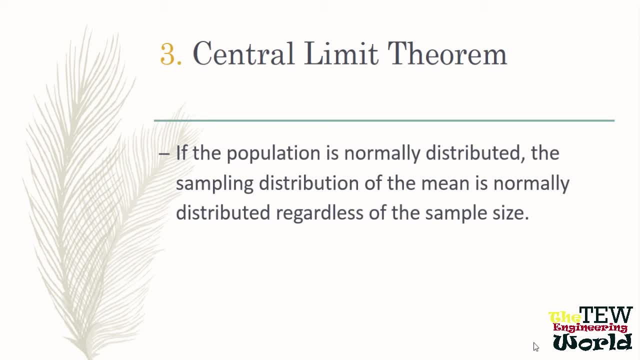 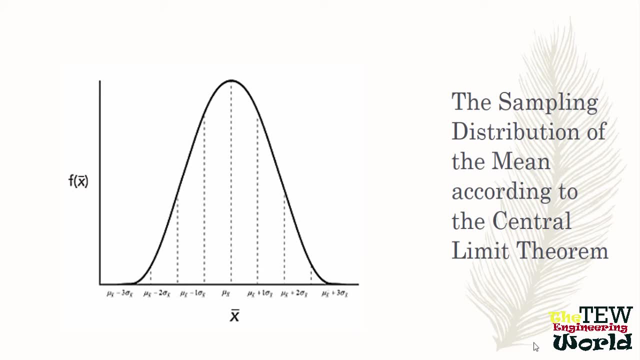 the mean is normally distributed regardless of the sample size. This is what the sampling distribution of the mean looks like according to the central limit theorem. It's a normal distribution with a mean equal to the mean of the population, and the standard errors are laid out across the x-axis. Here is an example of the central limit theorem at work. 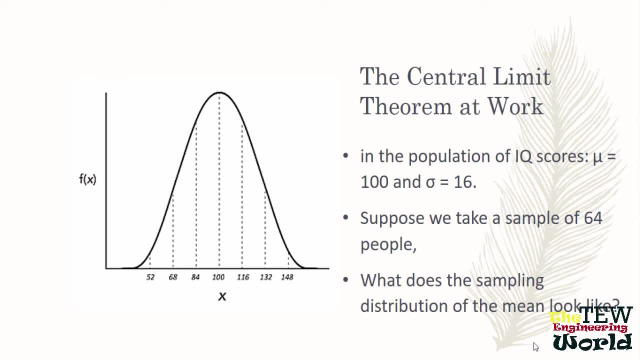 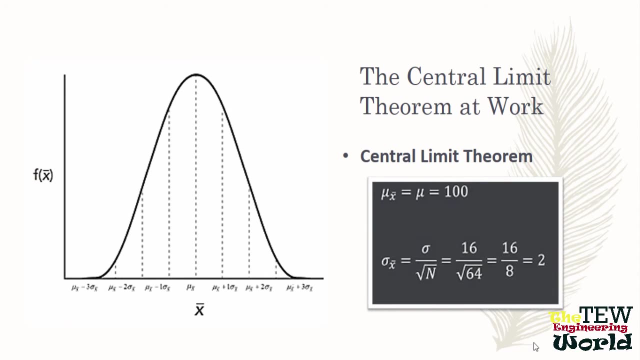 The population of IQ scores, with one version having a mean of 100 and a standard deviation of 16.. If we take a sample of 64 people, what does the sampling of the distribution of the mean look like? It looks like this: According to the central limit theorem, its mean is the same as the population mean, which? 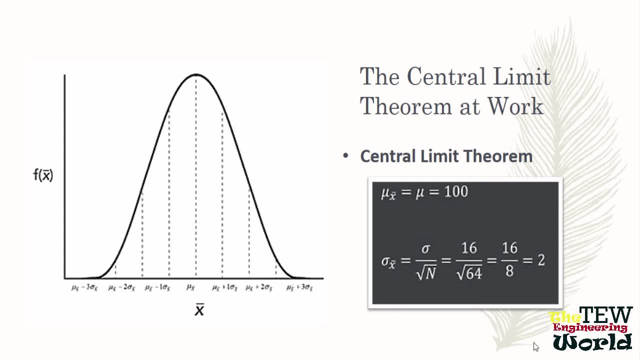 is 100, and its standard deviation, or the standard error of the mean, is equal to sigma divided by the square root of n, which is 16, divided by the square root of 64.. 16 over 8, which is 2.. And you can see those values laid out across the x-axis Now in the two preceding 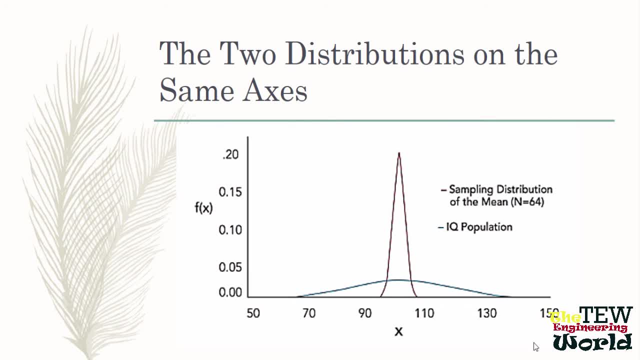 pictures. the population distribution looked very similar to the distribution of the sample, very much like the sampling distribution. That's because they appeared on different axes. This is what the population distribution and the sampling distribution look like when you plot both of them on the same set of axes. They are both normal distributions, but the 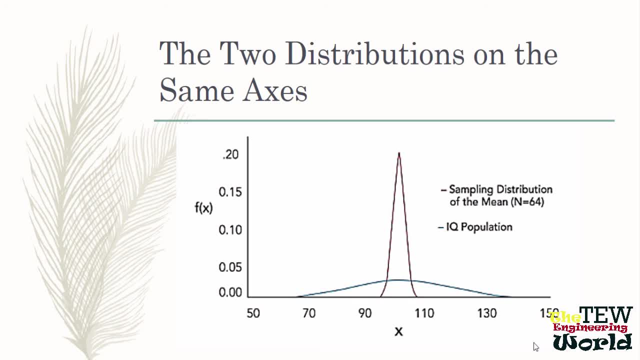 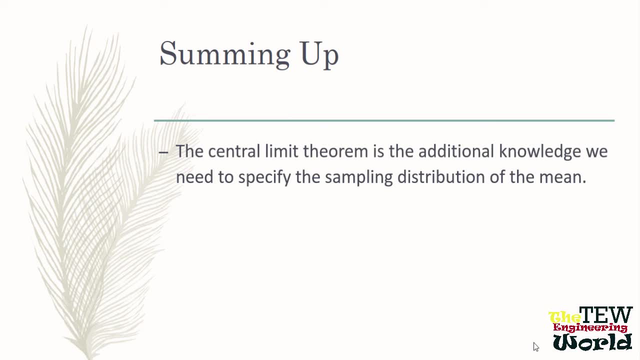 sampling distribution has a way smaller standard deviation. Summing up, the central limit theorem is additional knowledge. We need to specify the sampling distribution of the mean With data from just one sample. the central limit theorem can tell us the mean, the standard. 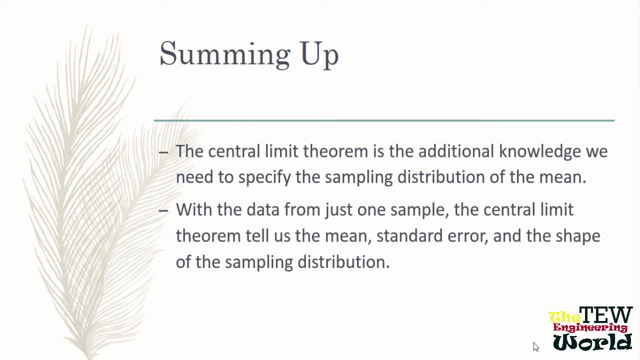 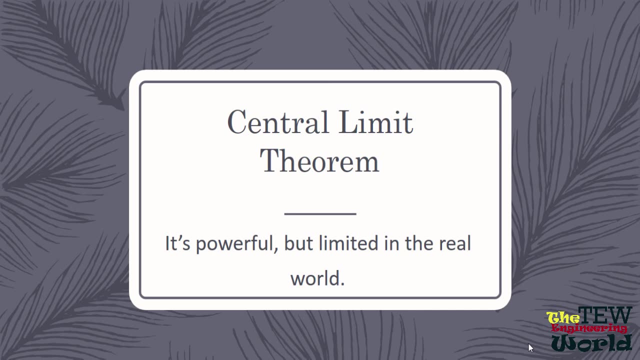 error and the shape of the sampling distribution, and that's a huge amount of information. We use this in estimation and in hypothesis testing. Let's look at a very useful family of distributions. It is called the t-distribution. Now we have looked at the central limit theorem. It's powerful, but it is limited in the real world. 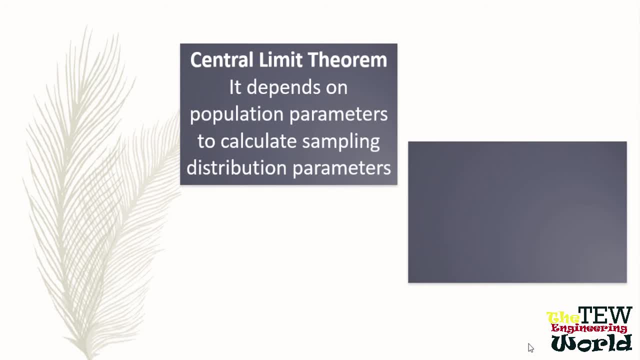 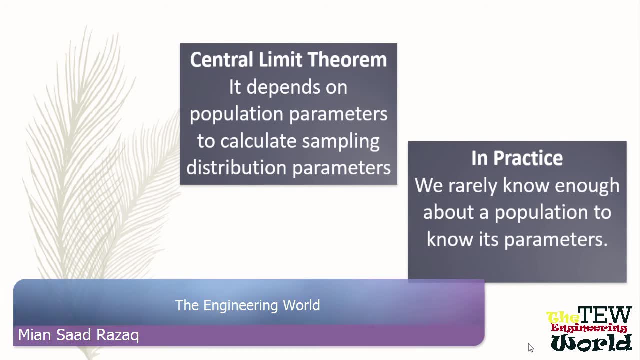 Why is that? The central limit theorem depends on population parameters to calculate sampling distribution parameters. In practice, we rarely know enough about a population to know its parameters. You could argue that if we knew enough to know a population's parameters, we would not have to gather any data. So we don't know the population and that's why we. 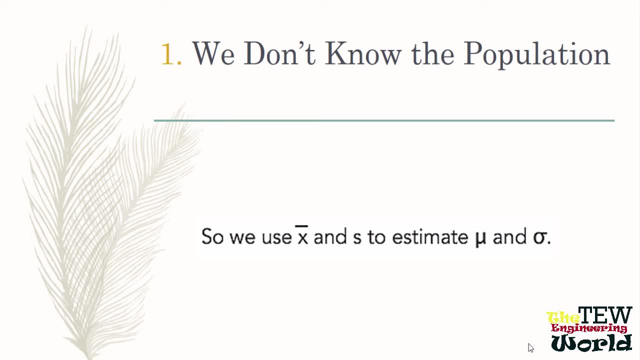 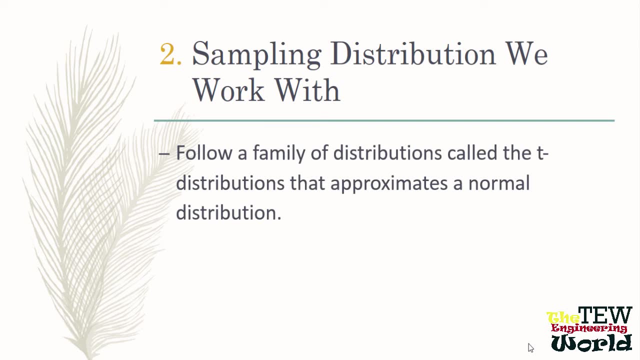 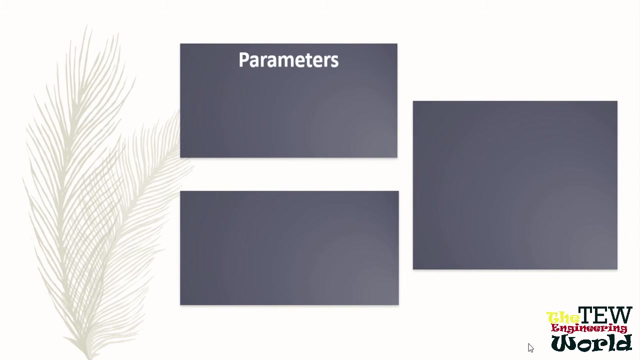 use x-bar and s to estimate mu and sigma. distribution that we typically work with follows a family of distributions called a t-distribution, and the members of this family approximate a normal distribution. How close a t-distribution comes to a normal distribution depends on the sample size As far as its parameters. 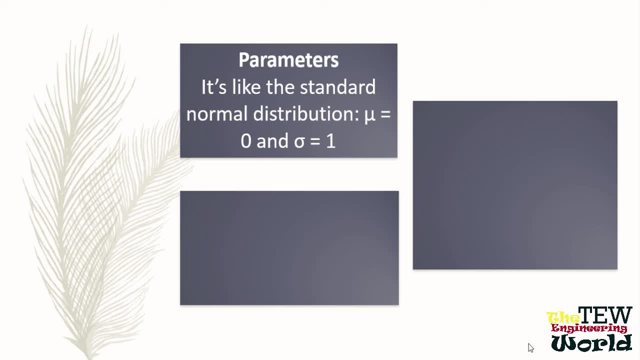 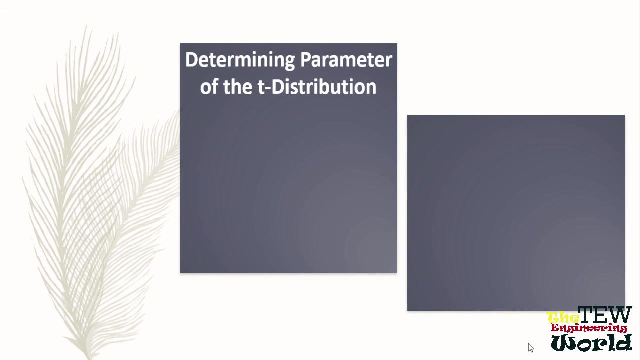 are concerned, it's like the standard normal distribution: Mu equals zero and sigma equals one. As for its shape, the probability density function is symmetric. Now, compared to the normal distribution, the probability density function is lower in the middle and higher at the tails, the extremes on either side. The determining parameter of the t-distribution. 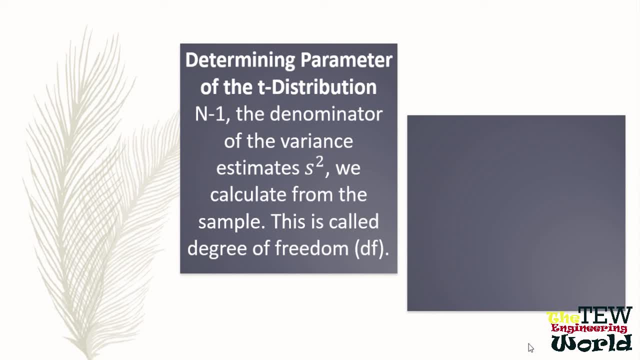 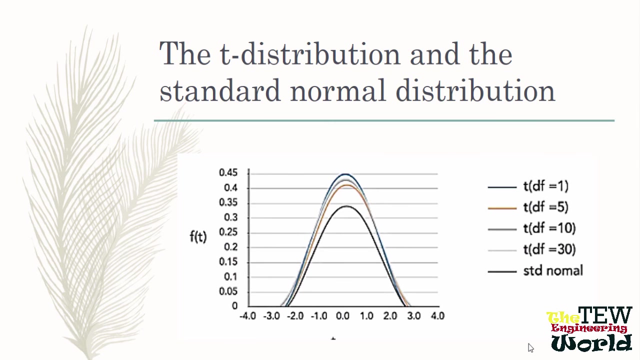 is n minus one, The denominator of the variance estimate s square we calculate from the sample. This is called degrees of freedom. If the degrees of freedom are 30 or more, then the difference between the t-distribution and the standard normal distribution is negligible. Here is what different members of the t-distribution 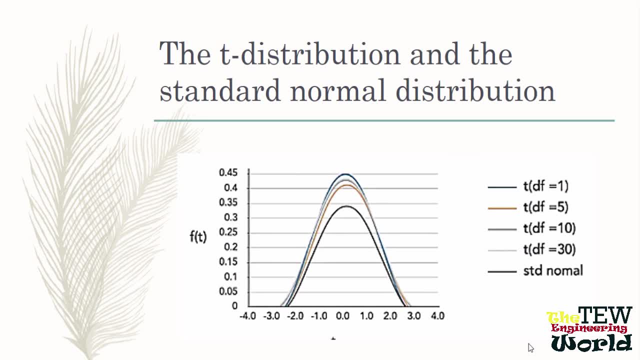 family look like in comparison to the standard normal distribution. As you can see, as degrees of freedom increases, the t-distribution gets closer and closer to the standard normal distribution. So, summing up, The central limit of the t-distribution is equal to the number of degrees of freedom. 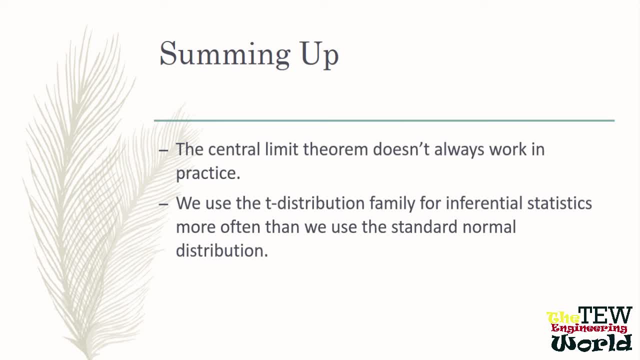 and the number of degrees of freedom is equal to the number of degrees of freedom. The distribution theorem does not always work in practice. You will find that we use the t-distribution family for inferential statistics more often than we use the standard normal distribution. The determining parameter for the t-distribution is called degrees of freedom. 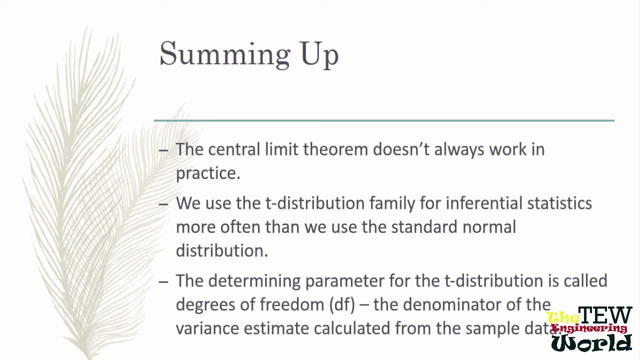 and it's the denominator of the variance estimate calculated from the sample data.